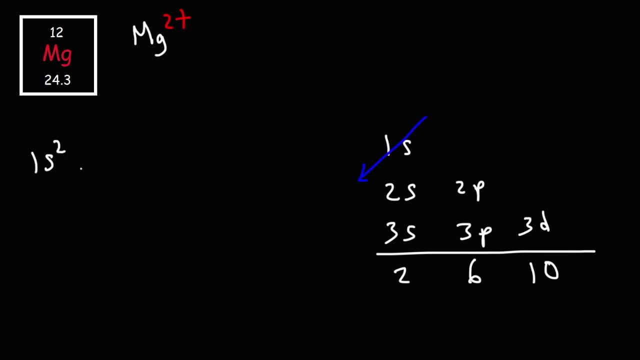 So we're going to start with this one. So first it's 1s, 2, and then we'll move on to 2s. So this is going to be 2s, 2, and then, after 2s, it's 2p, then 3s. p can hold up to 6,, and then 3s, 2.. So this is the electron configuration of the element magnesium. So if that's the case, what is the electron configuration of the ion Mg2 plus? All we need to do is take away 2 electrons. 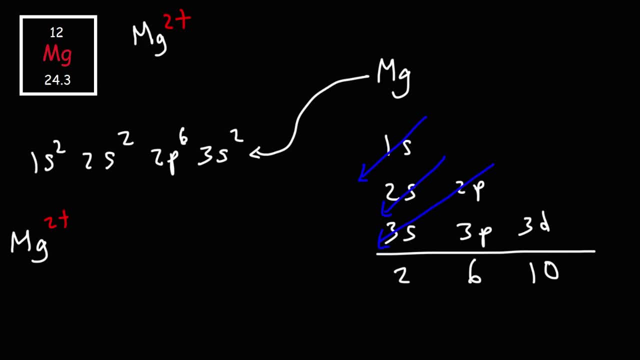 And what you need to do is take away the electrons from the highest energy level or the autumnal shell, which in this case, is the 3rd shell. So we're going to remove these 2 electrons, giving us a configuration of 1s2, 2s2, 2p6.. 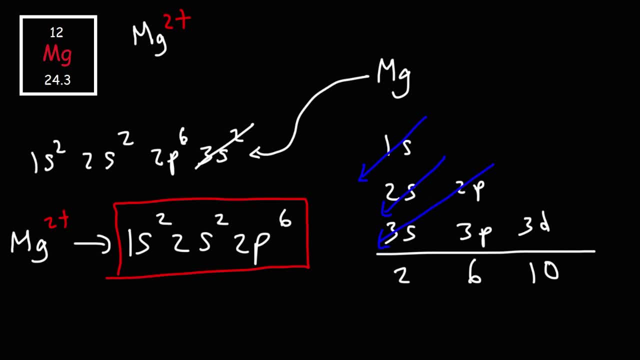 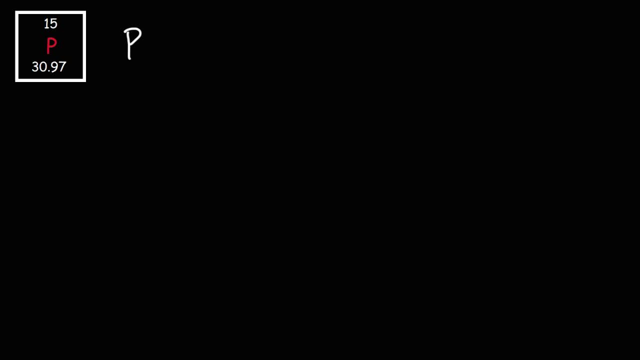 So this is the electron configuration of the ion Mg2 plus. Now let's move on to our next example. So this is going to be the phosphide ion p3-. Now there's something I want you to understand. Going back to the last example, we saw that magnesium had an atomic number of 12.. 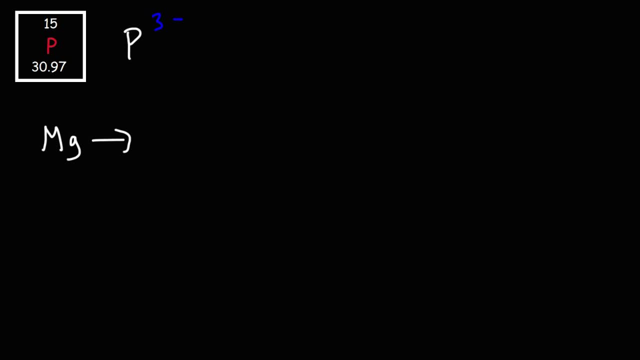 As an atom, this means that it has 12 protons and 12 electrons. Keep in mind, atoms are electrically neutral, so the number of protons and electrons are the same. So for magnesium. that's why the sum of the exponents of the electron configuration added to 12.. 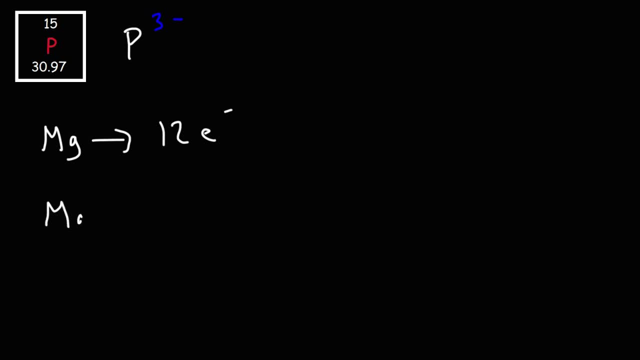 It's because it has 12 electrons. Now, when dealing with positively charged ions, the number of protons exceed the number of electrons. In Mg2 plus, there are 2 more protons than electrons, So we need to decrease the number of electrons by 2.. 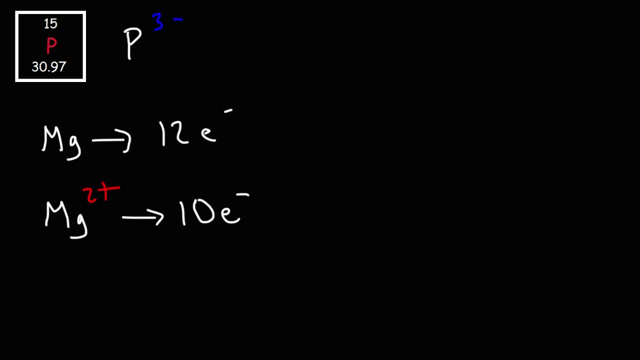 That's why the configuration was 1s2, 2s2, 2p6.. Because the exponents add up to 10.. The number of electrons Now? in the case of phosphorus, The atomic number, is 15, which means that it has 15 protons. 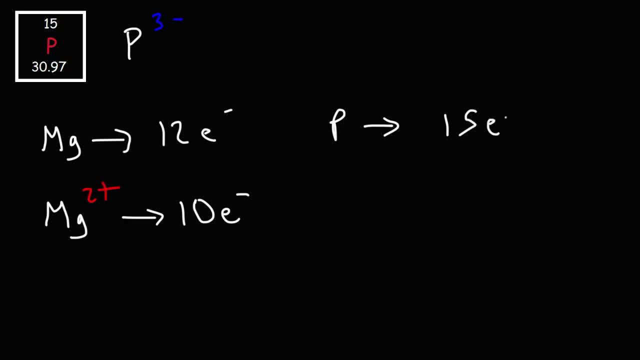 And as a neutral atom, it will also have 15 electrons. Now, as an ion, this situation is different. A negatively charged ion, also known as an anion, has more electrons than protons, So phosphide has 3 more electrons. 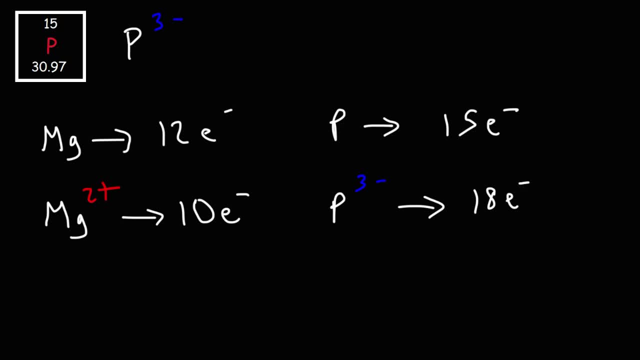 So what we need to do is we need to increase the number of electrons. need to do is, when we write the electron configuration for phosphorus, in order to write it for the phosphide ion, we need to add 3 to the number of exponents. so 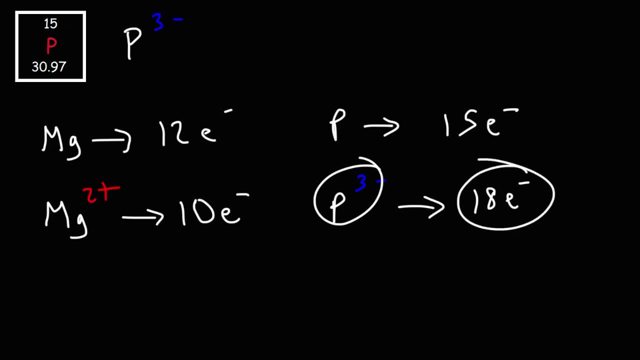 that the total is 18.. So, when dealing with positively charged ions, you need to decrease the number of electrons by the charge. When dealing with negatively charged ions, you need to increase the number of electrons based on the charge. Now let's focus on a problem at hand. Let's write the electron configuration. 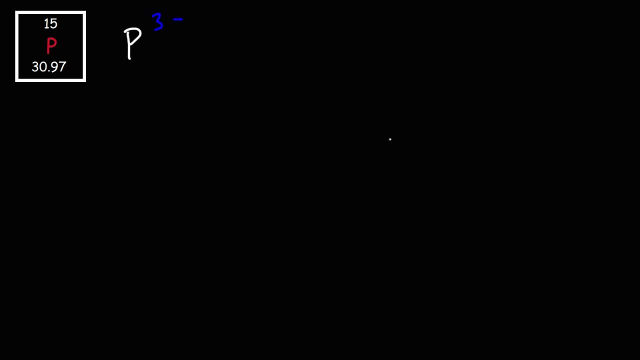 of the phosphide ion. So let's begin by writing the sublevels. Phosphorus is in the third row of the periodic table, so we only need to go to the 3s level. Keep in mind: the s sublevel can hold up to 2 electrons. the p sublevel can hold a. 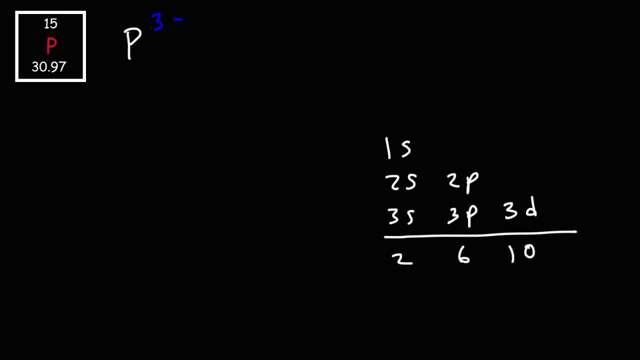 maximum of 6 electrons and the d sublevel can hold a maximum of 10 electrons, And we need to get up to 18.. But first let's write the electron configuration of phosphorus, which goes up to 15.. So it's going to be 1s2.. After that it's going to be 2s2.. After 2s it's. 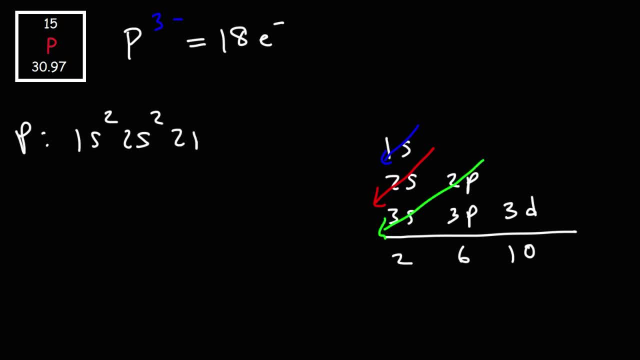 2p and then 3s, So 2p6, 3s2.. Right now we have a total of 12, if we add up the exponents, And then, after 3s, we're going to move on into 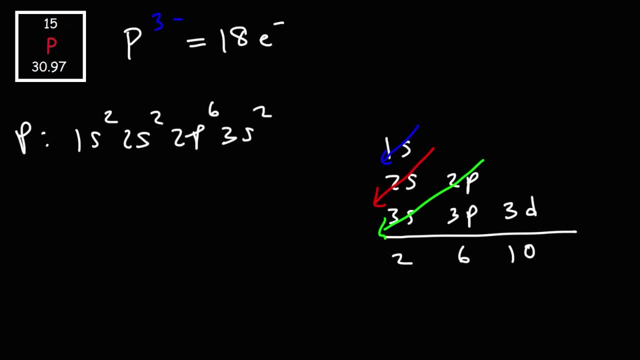 Let's undo that. So after 3s we're going to move on to the 3p sublevel and we're going to stop at 3p3.. So that's the electron configuration for an atom of phosphorus. Now for the p3- ion, we simply need to add 3 to this exponent, So the 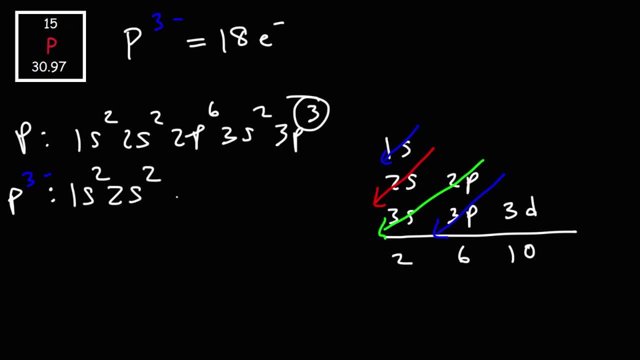 configuration is going to be 1s2,, 2s2, 2p6,, 3s2, and then 3p6.. So if you add up the exponents, the sum total is 18, because the phosphide ion has 18. 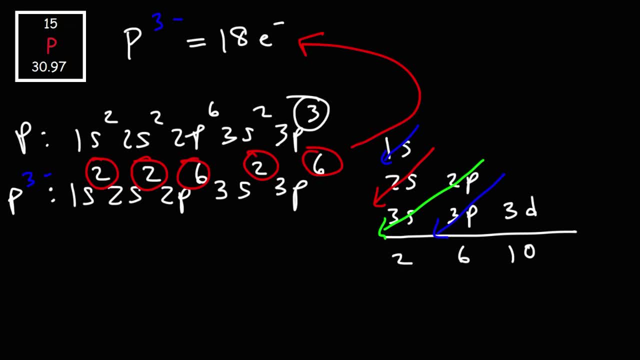 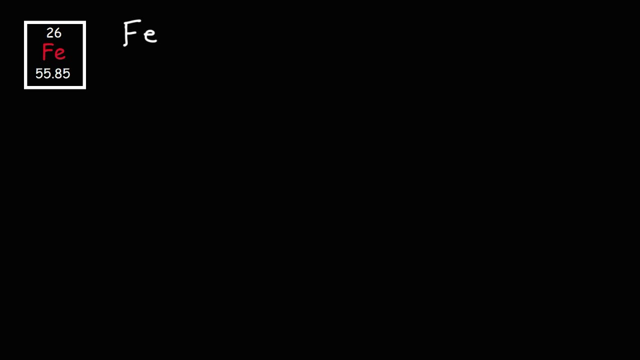 electrons in total. So that's how you can write the electron configuration of a negatively charged ion. You need to increase the number of electrons based on the negative charge that you see. Now for the next example, we're going to write the electron configuration for the Fe2 plus ion and also the Fe3 plus ion. Now, if you want to, 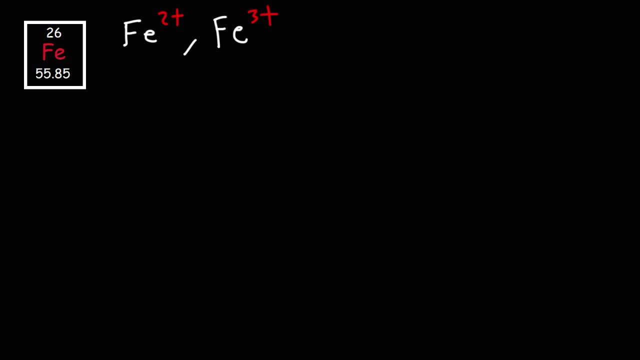 try this problem. feel free to do so. Go ahead, pause the video and work on it it. So let's begin by writing the sublevels. Fe is in the fourth row, so we're going to go up to 4s. 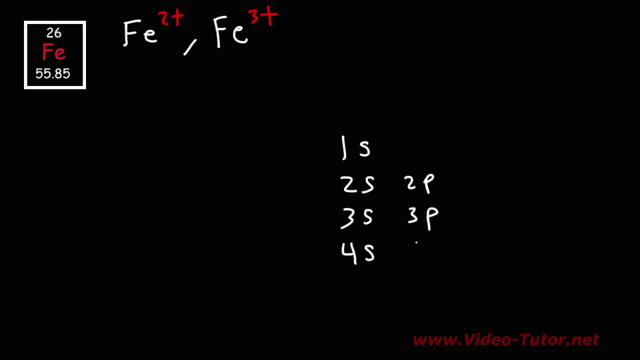 this time. S can hold up to 2 electrons, p can hold up to 6,, d can hold up to 10, and how much can F hold? Notice the pattern: this is increasing by 4, so 10 plus 4 is 14.. F can hold a maximum. 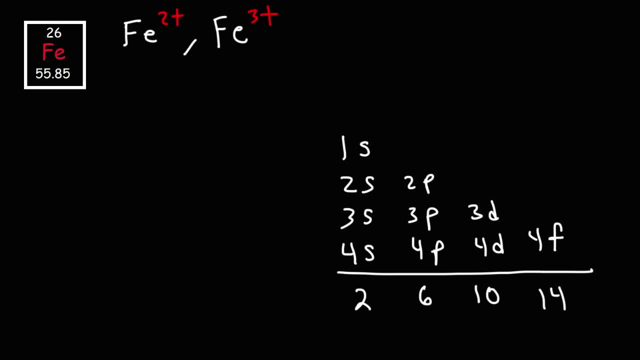 of 14 electrons. So first let's write the configuration for an atom of Fe. So we need to get up to 26.. So first we have 1s2,, next is 2s2.. And then after that it's 2p, then 3s. So we have 2p6, 3s2, and then it's 3p, then 4s. So 3p6, 4s2.. 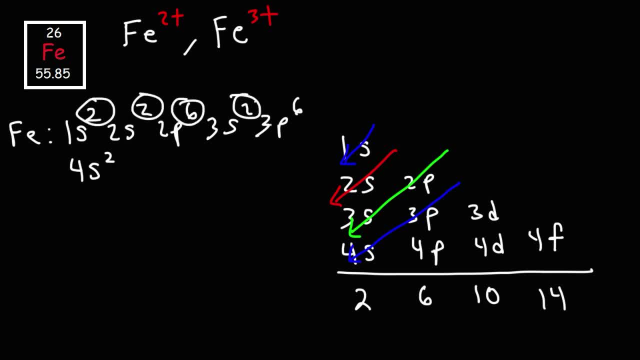 Right now. if we add up the exponents, this is 10, and then this is another 10,, so we have a total of 20 right now. So we need 6 more, So we can stop at the 3d level. d can hold up to 10, so we'll stop at 3d6.. This is the ground. 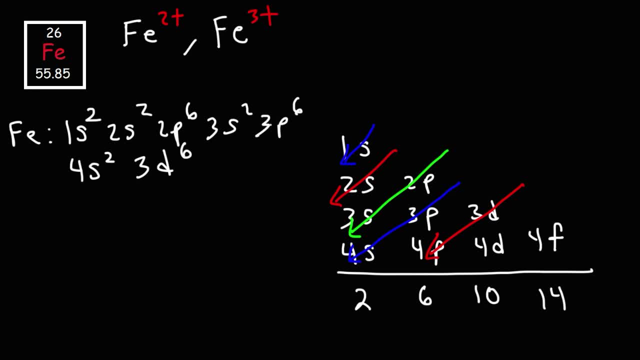 state electron configuration for an atom of iron, Fe. So now that we have that, we can now write the electron configuration for the transition metal ions Fe2 plus and Fe3 plus. So when dealing with cations or positively charged ions, you need to remove electrons. 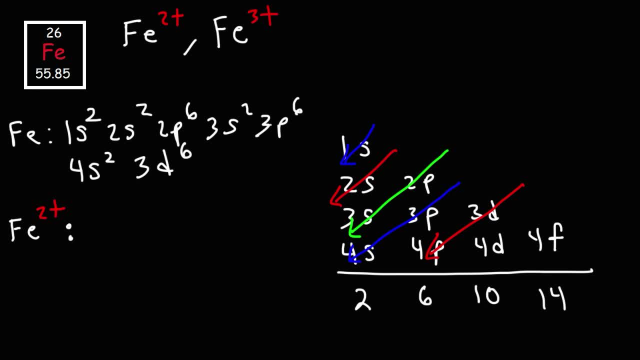 In the case of Fe2 plus, we need to take away two electrons. Now here's a question for you: Should we remove the two electrons from the 4s level or from the 3d level? When dealing with these type of problems, you want to remove the electrons from the highest energy. 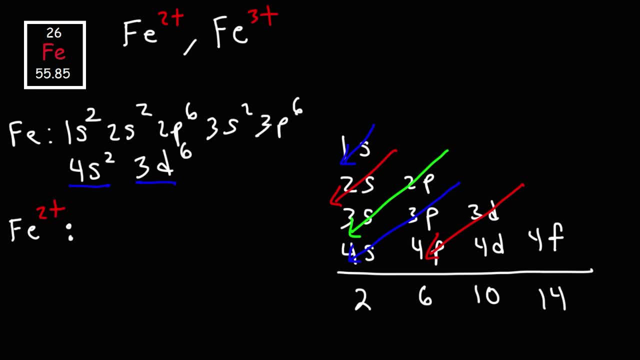 level, or the outermost shell, In this case from the fourth shell, before you move it from the three shell. So we're going to take away the two electrons from the 4s level As opposed to the 3d level, So we'll be left with 1s2, 2s2, 2p6,, 3s2, 3p6.. Now, at this point, 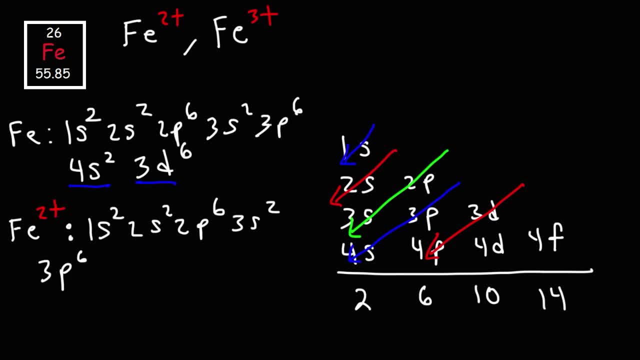 you can either write 4s0 or you can just omit it together. Just to keep track of things, I'm going to write 4s0 and then 3d6.. So that is the electron configuration of the Fe2 plus ion. 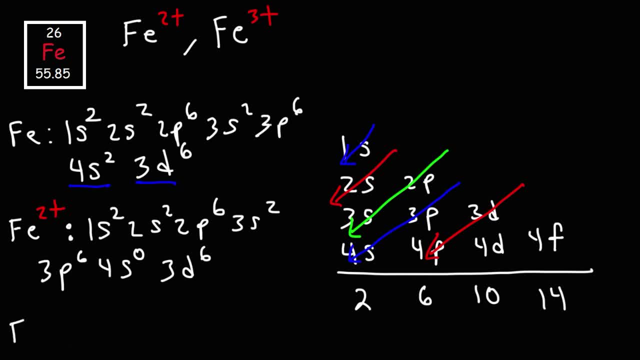 Now let's move on to the last ion, Fe3 plus. Now, in this case, we need to take away three electrons as opposed to two, And we're going to start by removing the electrons from the highest energy level. So the first two electrons we're going to take are the 4s2 electrons, And then we're going to 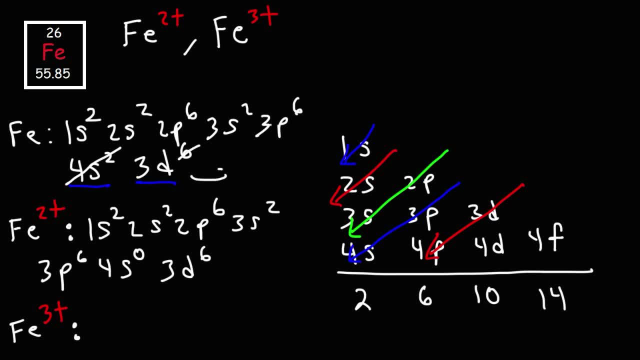 take one from the 3d sub level. So instead of having 3d6, we're going to have 3d5.. Thus the electron configuration of the Fe3 plus ion is 1s2, 2s2, 2p6, 3s2, 3p6, 4s0, 3d5. 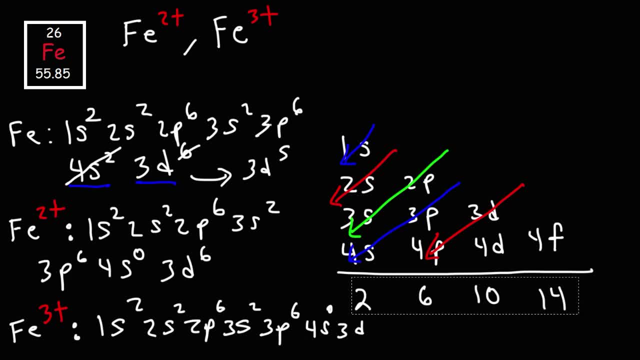 Let me delete these things, since they're getting in the way. Okay, now notice the total number of. let me say that again. Notice the total number of electrons in Fe3 plus: It's 26 minus 3, which is 23.. 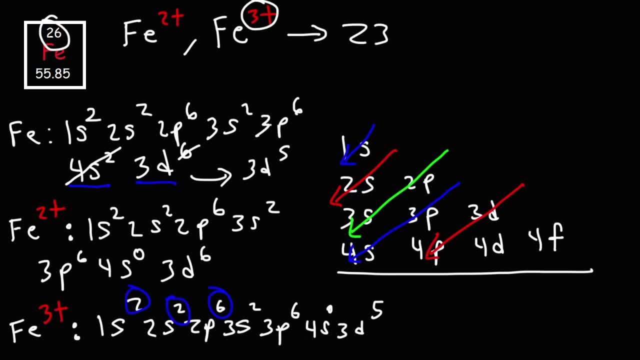 So when checking your work, the sum of these exponents must add a 23.. Right now this is 10,, 12,, 18,, and then 18 plus 5 is 23.. So this is the ground state electron configuration.